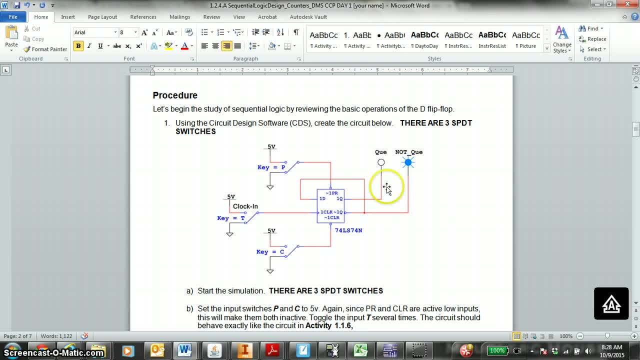 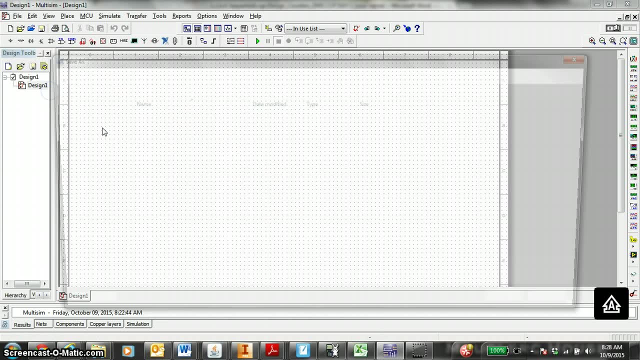 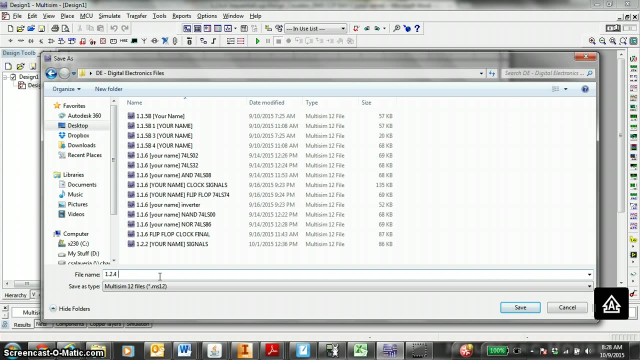 A 74.. LS 74 and clock two probes. So you open a new design. I would file save as this immediately. File save as into your Digital Electronics folder 1.2.4.. Your name. So you're building a library of files for reference. 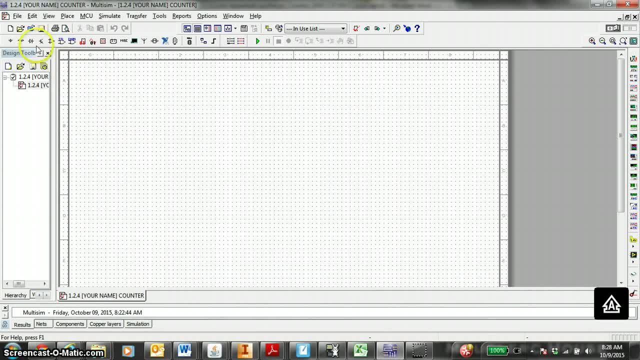 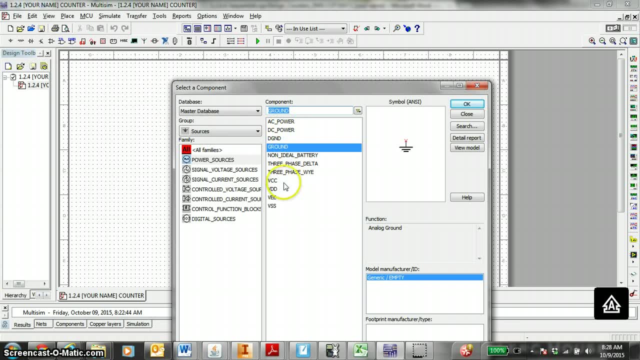 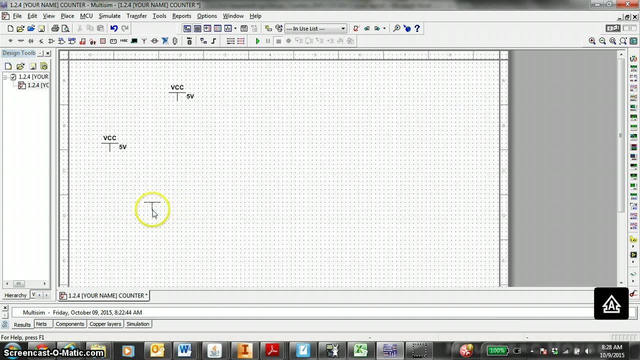 Call this counter. So no, it's yours. We need three 5-volt VCCs, So you could put three of these where appropriate. We need three digital grounds, not three digital undergrounds: 1., 2., 3.. 3., 4., 5., 6., 7., 8., 9., 10., 11., 12., 13., 14., 15., 16., 17., 18., 19.. 20., 21., 22., 22., 23., 24., 24., 25., 26., 27., 28., 29., 30., 32., 33., 34., 35.. 36., 37., 38., 39., 40., 41., 42., 43., 44., 44., 45., 46., 47., 48., 49., 50., 51.. 52., 53., 54., 55., 56., 57., 58., 59., 60., 61., 62., 63., 64., 65., 66., 67., 68.. 79., 68., 69., 70., 63., 63., 63., 64., 64., 63., 64., 65., 65., 66., 67., 68., 69.. 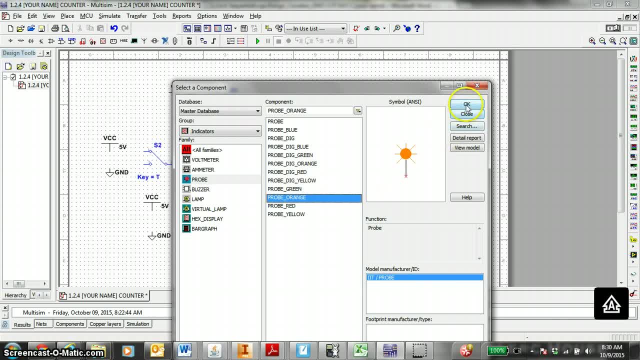 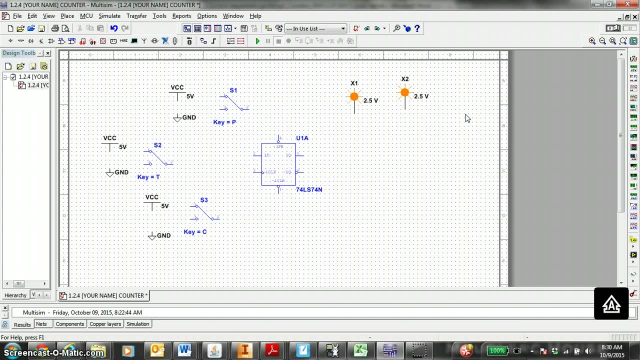 79., 68., 62., 62., 63.. the line I orange. I want to these here close and then I think you wire this up. so let's see where you click is where it you create like the wire. so I think this one goes to clear clock in. this is your. 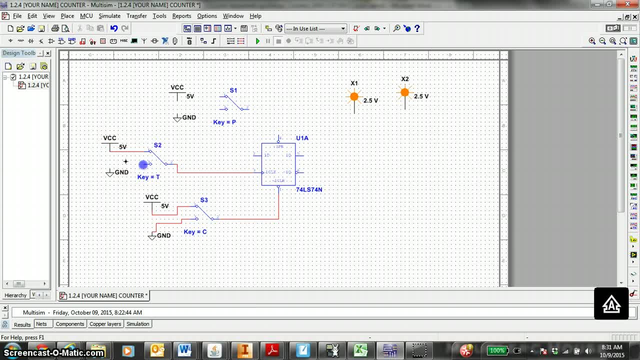 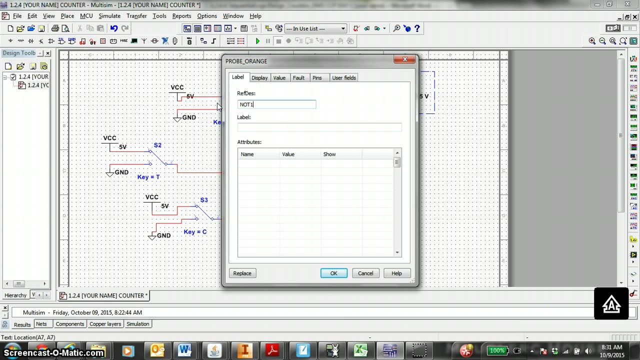 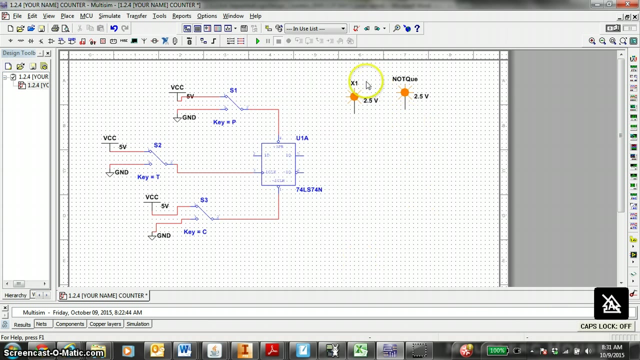 timer goes to that. you got to connect it to the hot in the ground, connect the switch to the low and the high signal. I believe this one goes to preset the top. let's make this. let's rename this not not Q. we call this koi Q quay. so this one gets connected to here. so the knot goes. 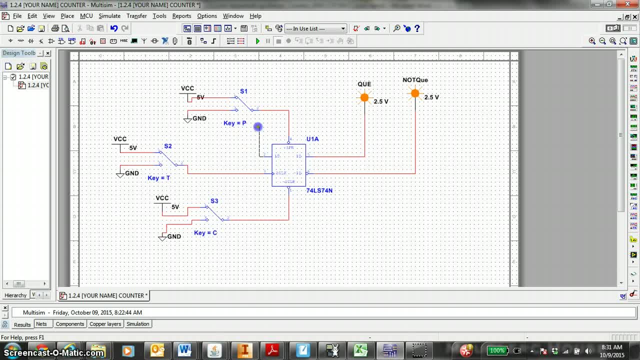 with that tilde. that means not, and I believe this one comes all the way around. pull around. that might look sloppy, but that's alright. bam boom. it says: make sure switch P to ground and C to 5 volts of. C is on, 5 volts, P to. 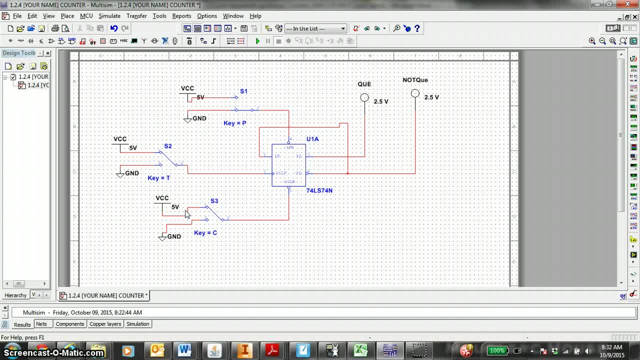 ground. let's run it. toggle this, see many times. so hopefully you figure out what's happening when you're pressing the T switch. step E set the input switch P to 5 volts. so we're gonna make that high. switch the clock. CLK to ground, get it to output. so I go switch several times, see. 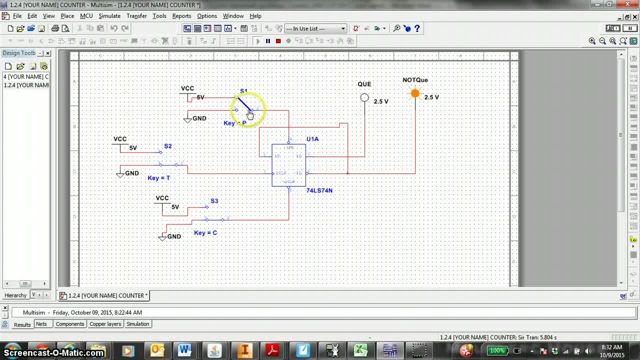 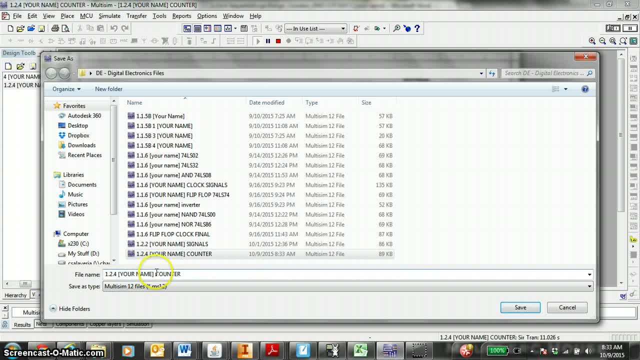 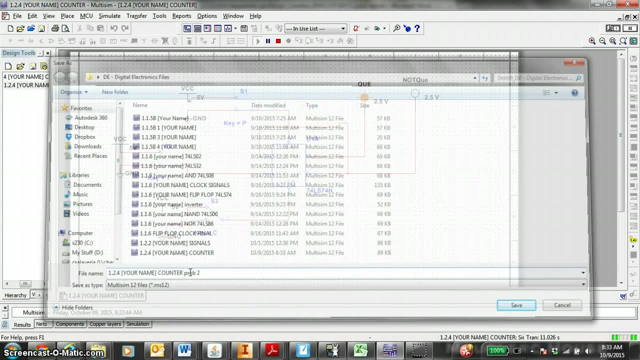 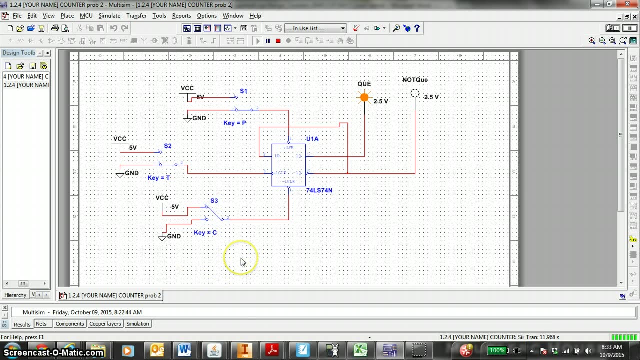 save as. let's call this next one: 1.24, your name counter, problem T. so we're looking at this binary counter over here. we're adding a second: 74 LS, 74 N, I think we can. can delete this switch. Oh, we have to turn off the simulation. Let's delete this. Delete this. 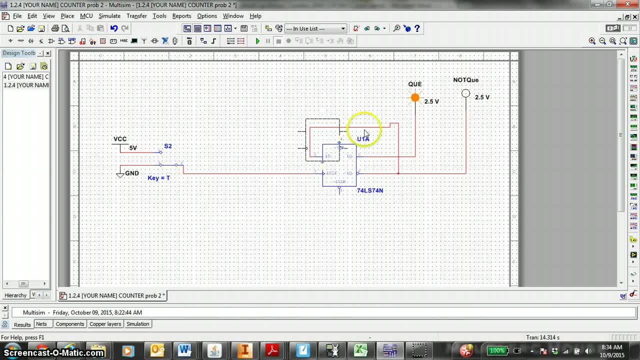 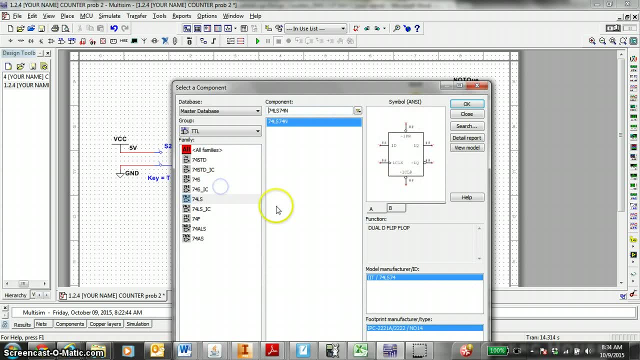 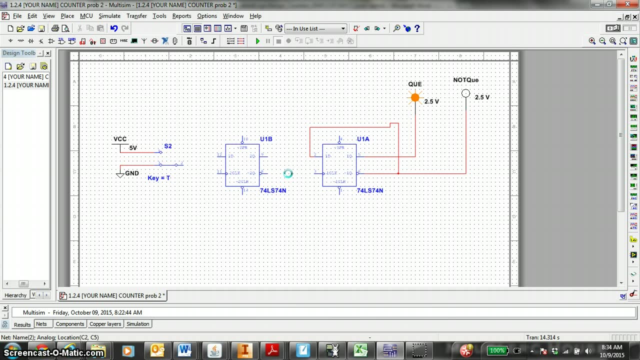 TTL. Okay, Let's use the B gate. Cancel, Close. Let's delete this wire. All we're going to have is a clock in T signal. We wire it up accordingly, so I would delete all these wires. The A gate's on the right, B gate is on the left. We need a second VCC. 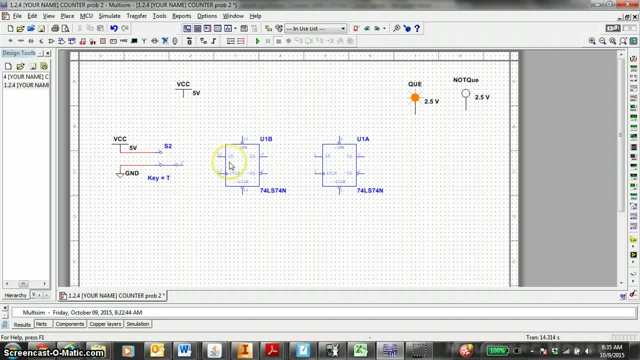 All right, Let's just follow the diagram. Knot Q on this. one goes to clock. here VCC powers the preset and it powers this guy here, This D here would go all the way around To this wire. here Q from the left gate goes to the probe. 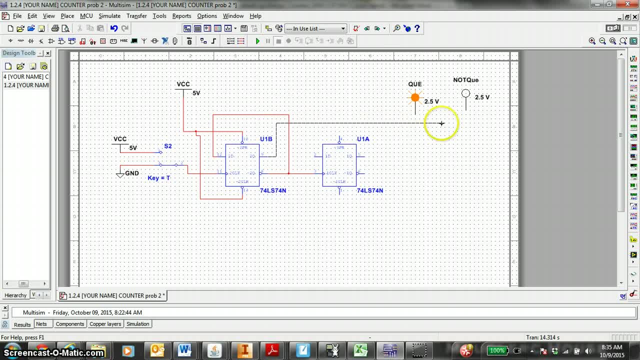 Yes, it does get confusing. Just go like this: Boom. I think I wired the B gate correctly. This PR also gets connected to the 5 volts Hot over here. This D over here gets connected to Knot Q on the other side. 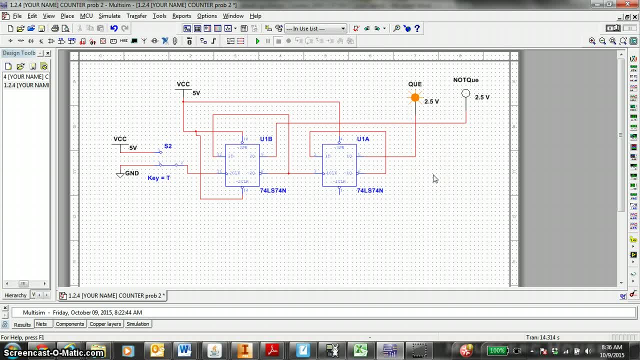 This Q gets connected to this probe And we definitely need power over here like that. All right, So hopefully you did this correctly. Provide screenshot of your multi-symbolo for three points. It's on the word document: Print screen Control V. 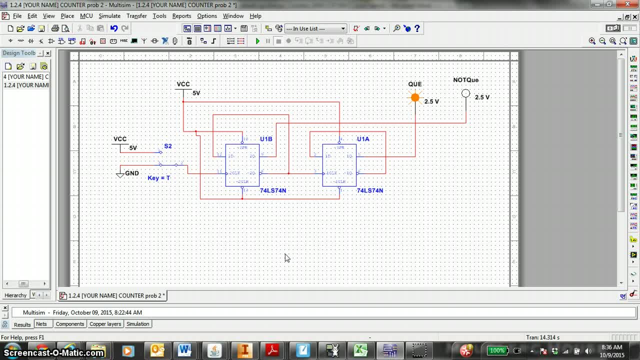 Toggle the first flip-flop changes only when the clock in goes out from low to high. I'm just reading the directions 3B: Toggle the input clock in switch T until both outputs A and B are low And T switch is low. 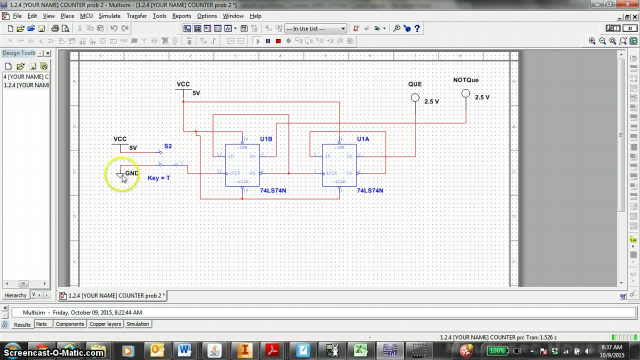 You've got to keep going. There you go. We want switch T on ground on ground and both off. so you might have to figure it out not there but there. and remember, one cycle needs to toggle from low to high, back to low, so one cycle, oh. 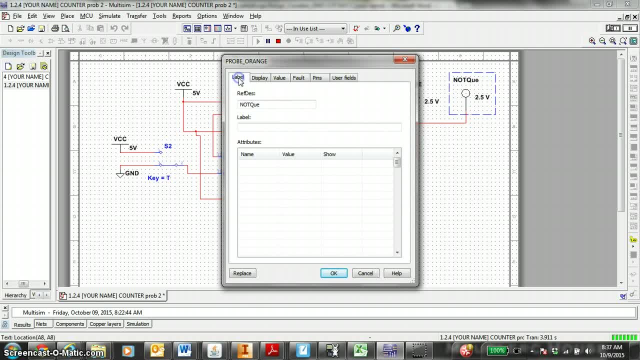 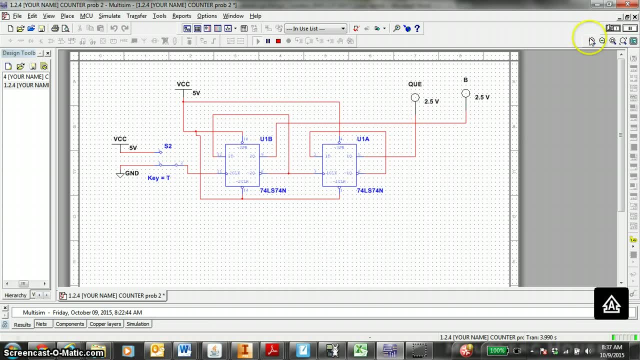 you might want to rename this B so you don't get confused. B call this now. simulation is running, of course, label a, let's run it. one cycle is that? figure it out when you fill in electronically on your Word document. another cycle on off. another cycle, high, low, another cycle. 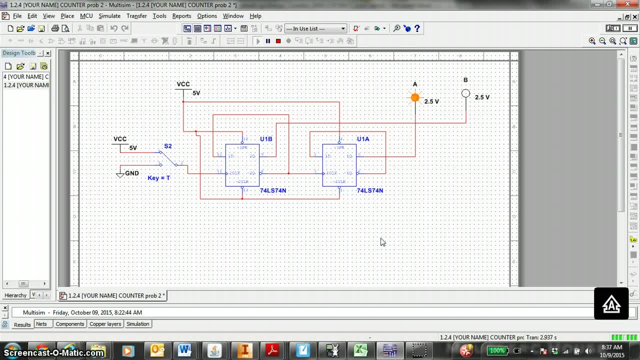 high, low. hopefully you get your nine cycles and know how to count in binary. I would save this, turn off the simulation and we move on. okay, make sure the simulations off and then I would save it and then file save as oops. file save as we're on still. 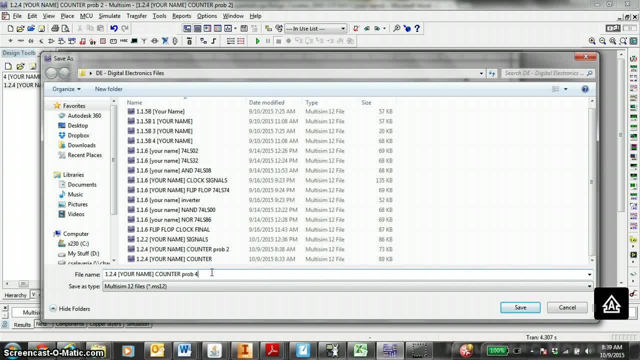 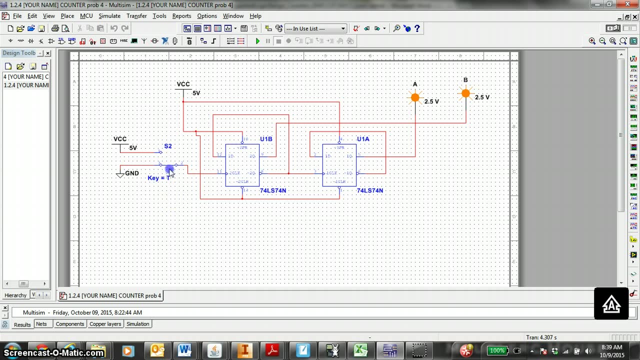 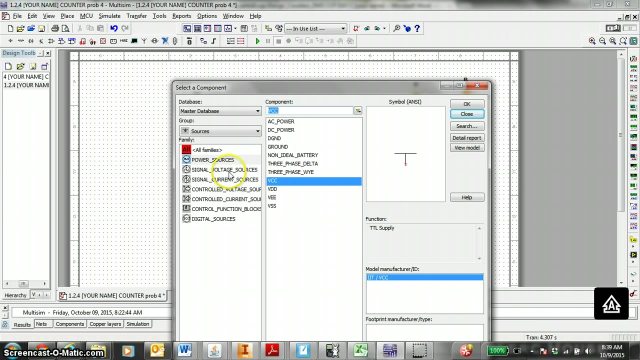 activity one, point two, point four. now we're on problem four. we're gonna use an oscilloscope and a clock voltage with what we got. so problem four: make sure you're off the simulation- I think you delete this guy- and then we need a signal voltage, source, clock voltage. good, put it right there. oh we. 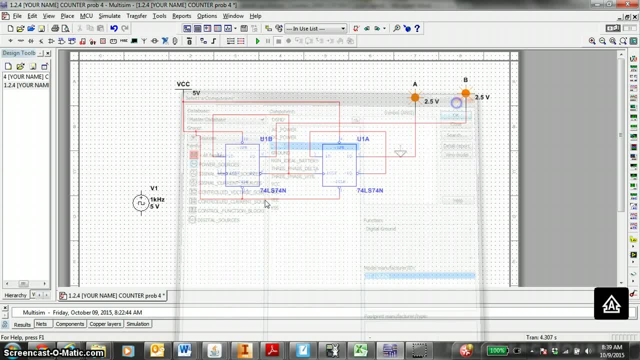 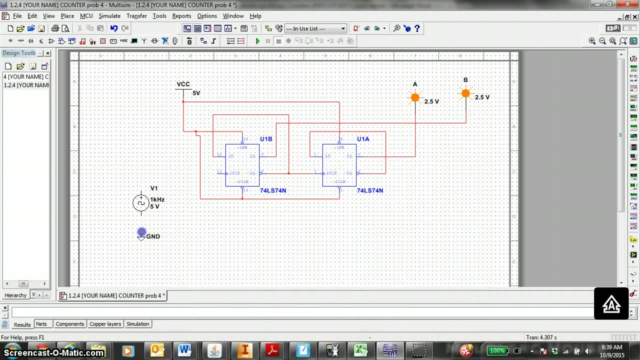 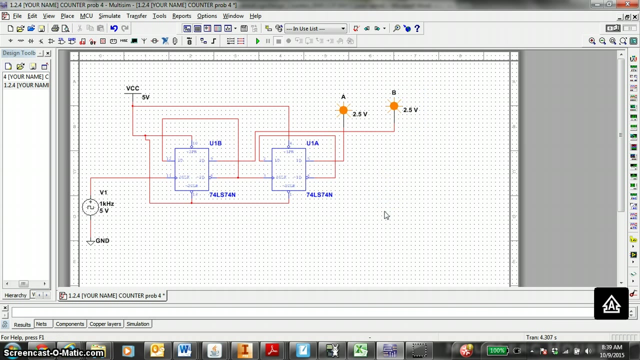 need a digital ground as well. so power sortir digital ground. okay, kind of goes there. sure, close, let's connect this here, connect this to the input. might want to slide everything over a little bit. slide that over, hopefully it doesn't ruin it. then we need the four channel oscilloscope.